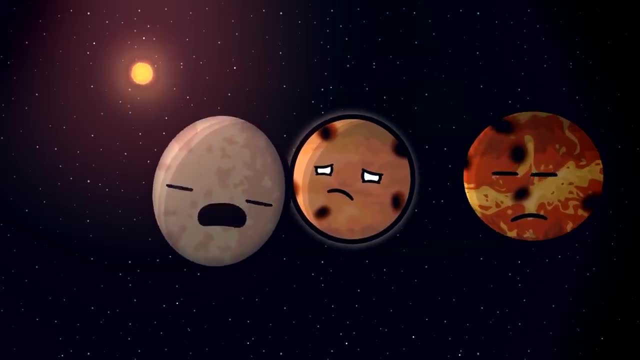 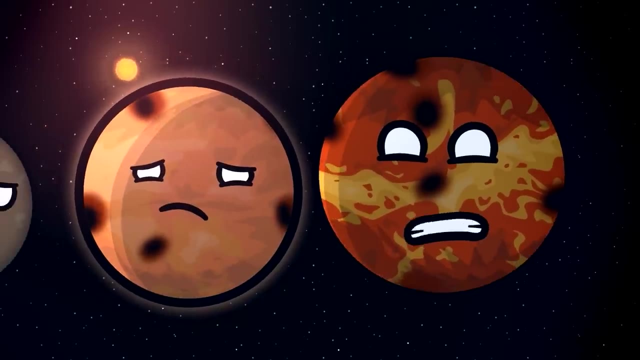 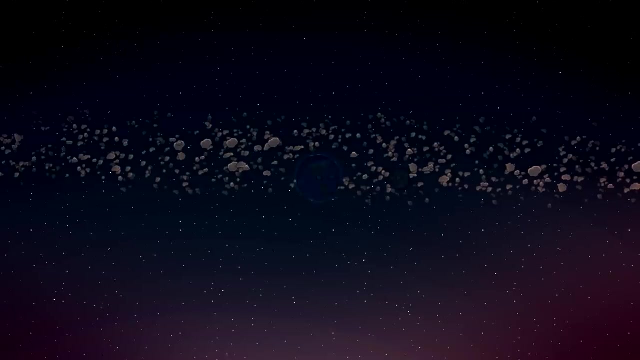 I hope Earth is okay. I can't believe you went to the asteroid belt alone. Yeah, the two of us could barely make it out alive. That's it. We must Wait. That's them. You're okay. And not a single asteroid crater on you. 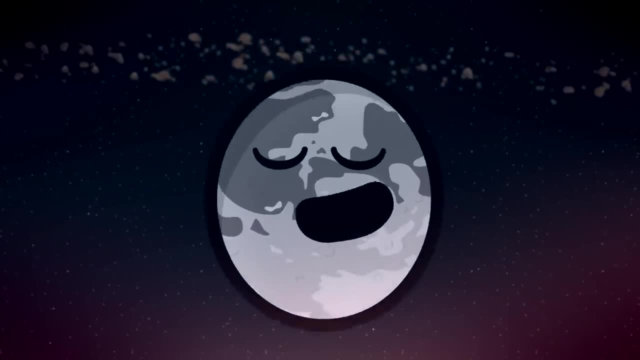 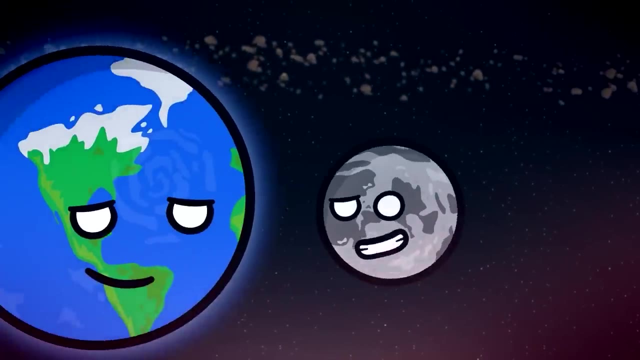 How Well the Earth spoke to the moons and calmed things down. Come on, Pluto and Sharon were the ones who convinced them. not me, Yeah, but you apologized to Titan That turned the tables on the whole situation. Anyways, let's not get lost in the details. 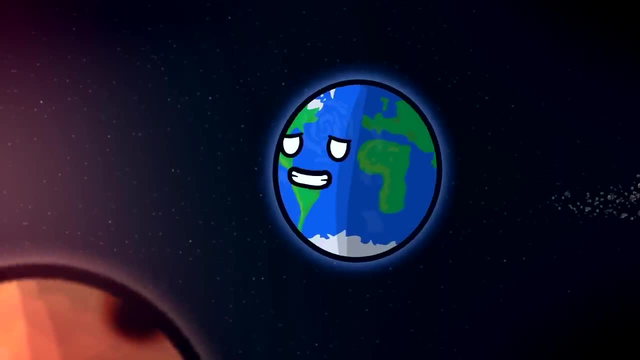 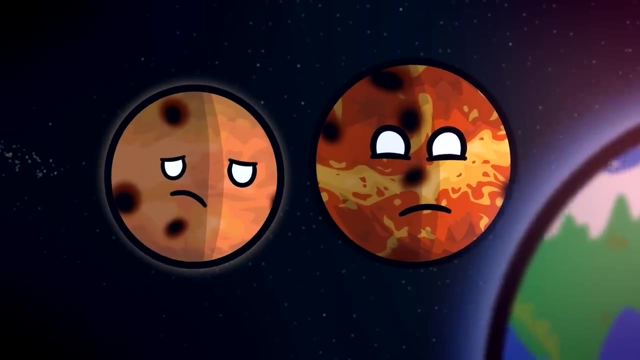 What's important is that it's all over and we can go back to normality. Oh, and I'm sorry, I wasn't a good friend to either of you. I made everything about myself and I see that now. Thank you for defending me, despite how bad I was. 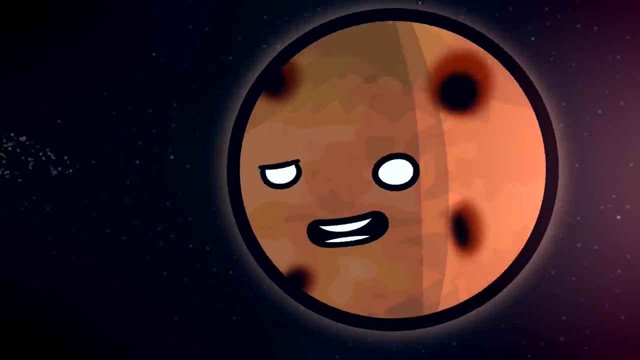 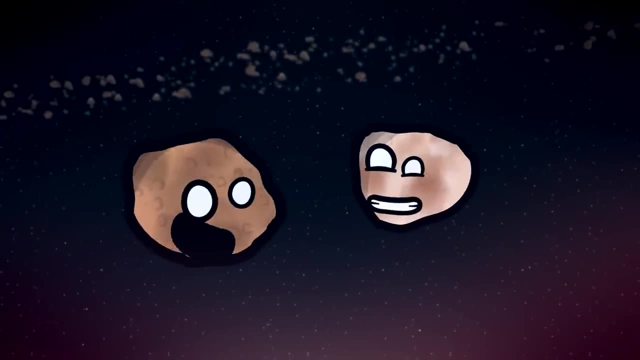 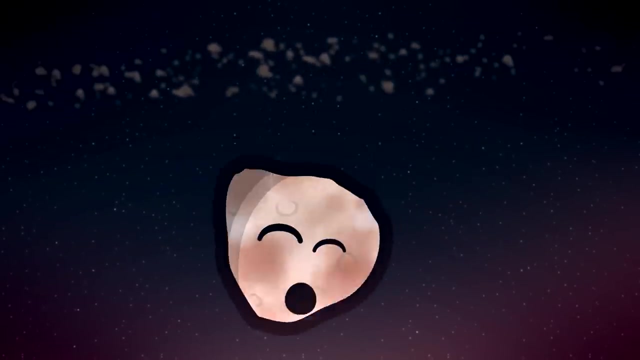 Earth. I Hey, if it isn't my moons. Tell him, Phobos. Tell him how brave we were. We were so brave Mars. We almost stopped an asteroid that was heading towards the Earth. Wait, almost, Yeah, but the Earthlings nuked it. It was so cool. 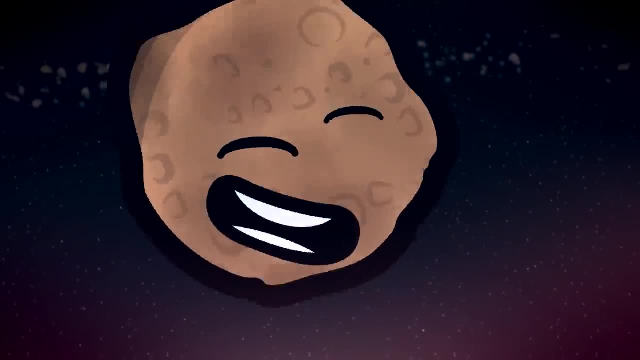 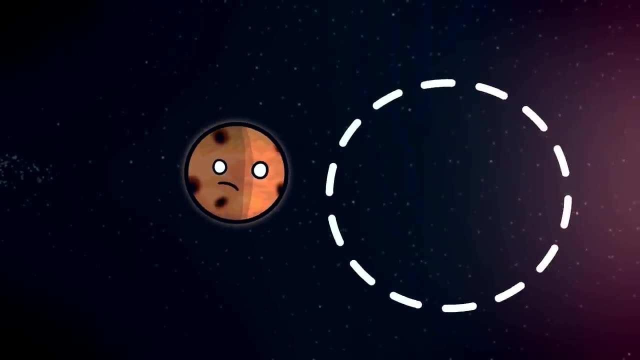 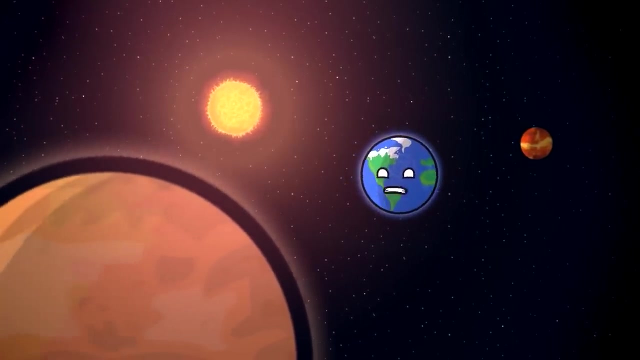 I still see the huge ball of fire when I close my eyes. Wow, Seems like we missed the whole adventure Earth. why don't you tell us the whole? Oh, Hey Mars, Hey Earth. I was Going towards Venus, right? 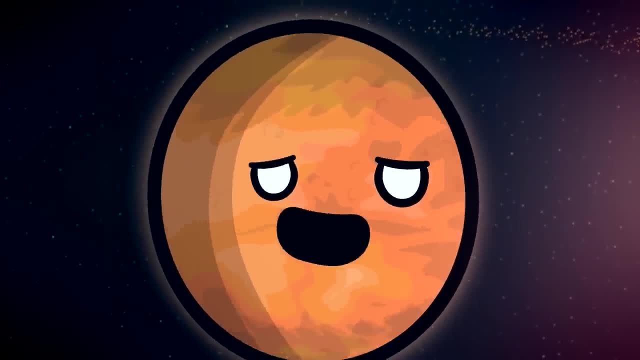 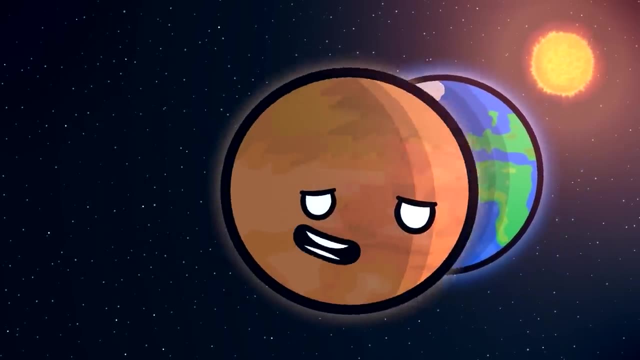 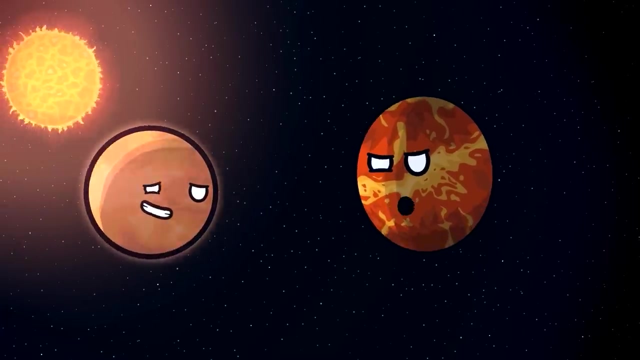 Right, We're friends now. Good old Venus. Mr Mr Venus, Just keep an eye on the sun so he doesn't shoot a solar flare at us. Yeah, gotcha pal, See ya pal, What was that? 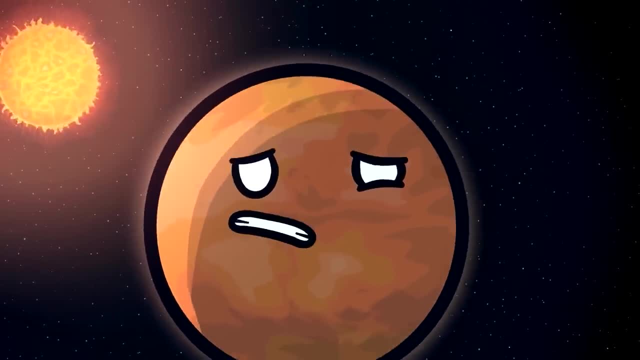 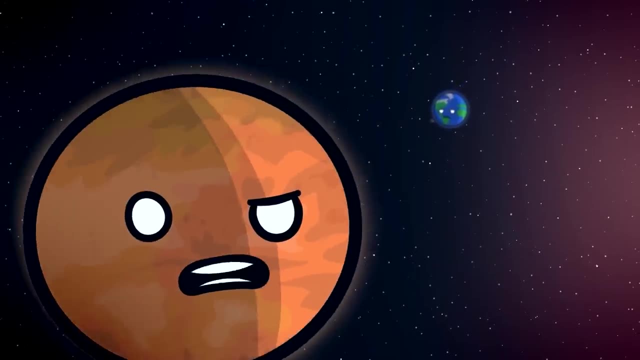 The most awkward talk I've had in In 4.6 billion years. Ugh, Is it that bad? It's like I don't even know how to talk to him. I honestly had given up on the Earth ever apologizing to us, but now like 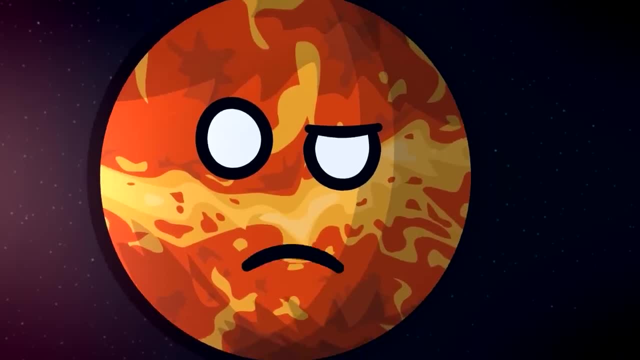 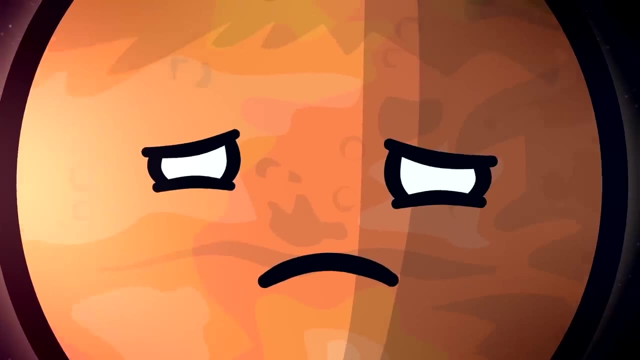 What do we do? I don't know. Last time we saw him he was insufferable And now he's like all introspective. We definitely missed something. That's it. You're a genius, Venus, Venus. 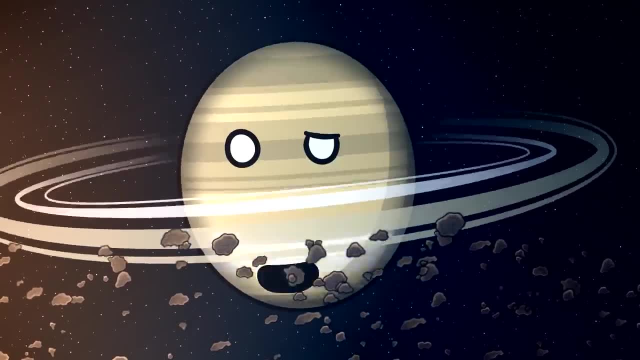 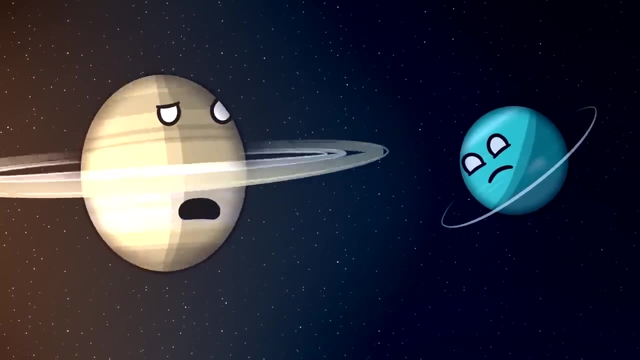 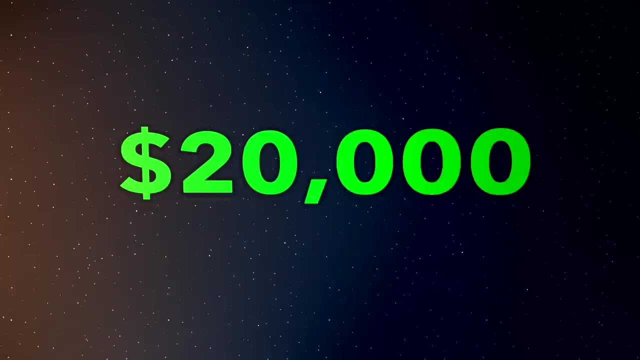 Venus the genius Looks like the rocky planets are having their fun. Hey, what are you doing, mate? You're gonna miss the scavenger hunt. Scavenger hunt, Yeah. Opera, the sponsor of today's video, is launching an awesome scavenger hunt with a reward pool of $20,000!. 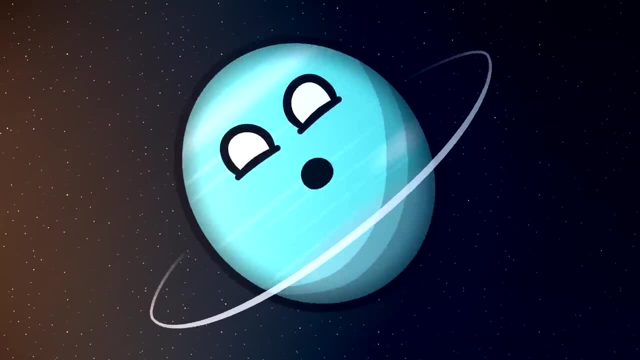 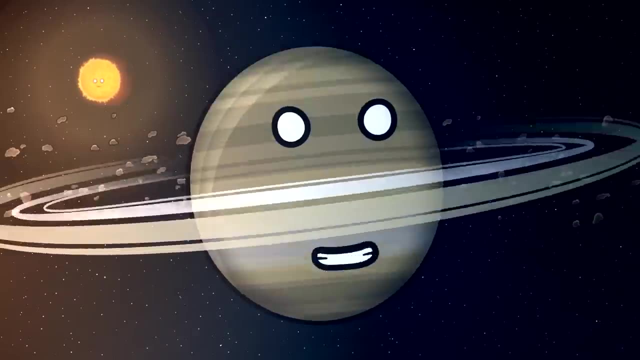 Whoa Wait Opera? Yeah, you know The internet browser with cool things like crisper videos, sidebars with tons of helpful tools, yadda, yadda, yadda. Yeah, These guys sponsored us some time ago, didn't they? 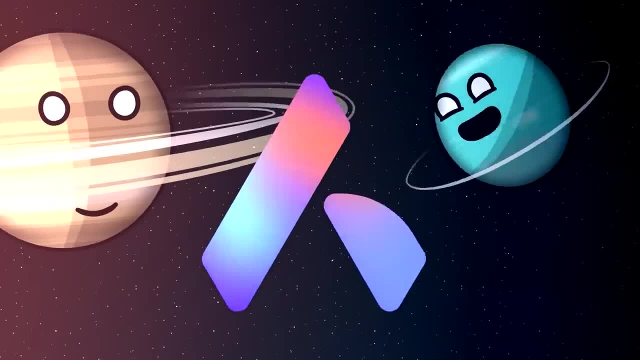 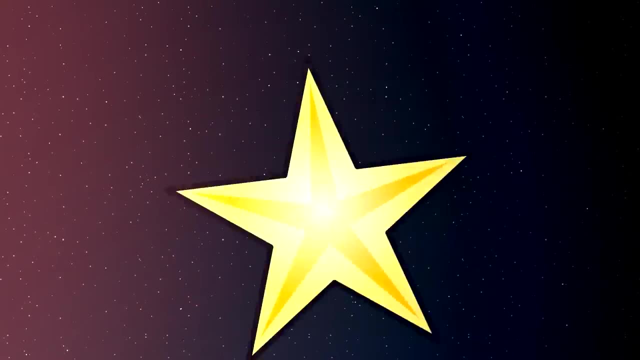 They did, but now they have their own AI named Aria, And she's in charge of the entire scavenger hunt. Basically, you follow the clues, solve the riddles Aria gives you, and then you could be one of the winners. 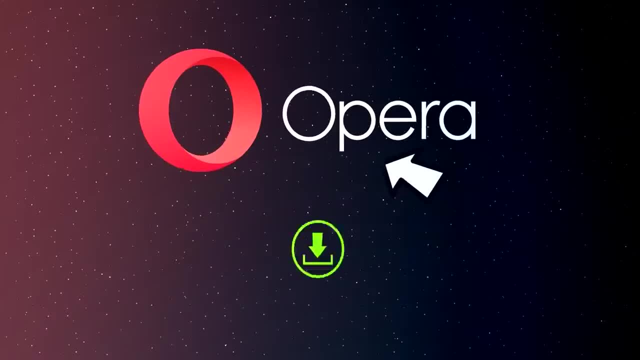 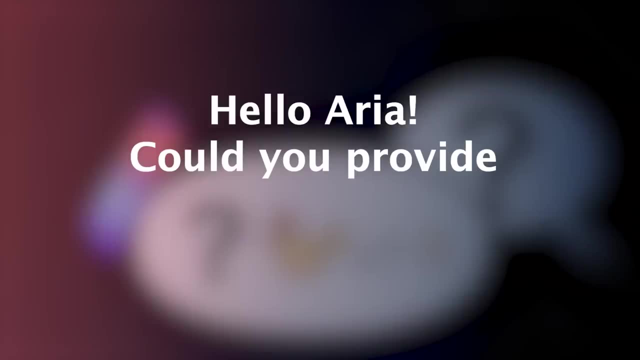 Well, come on Uranus. How do we even get started? First, you download Opera and activate Aria. Second, ask Aria for a clue with the prompt: Hello Aria, Could you provide today's clue for the Aria scavenger hunt? 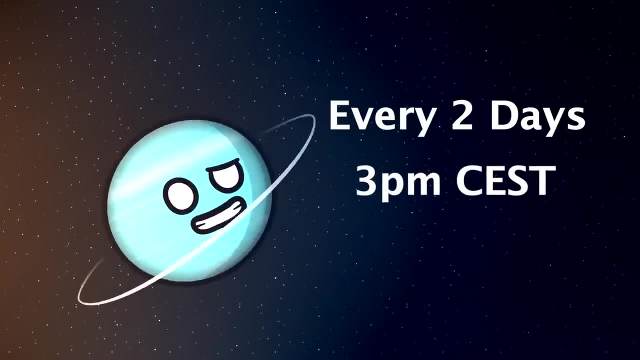 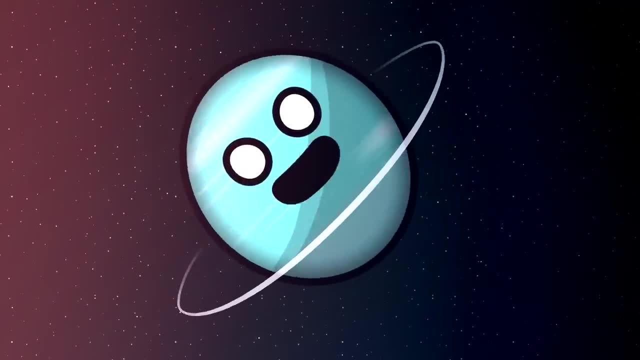 She will have a new one every two days at 3 pm CET, starting from the 3rd of April. Third, you solve the riddle, verify it with Aria and submit your answer. And step four: be the fastest scavenger and win the money prizes. 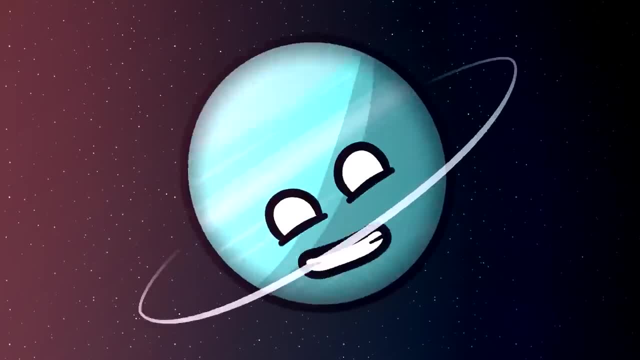 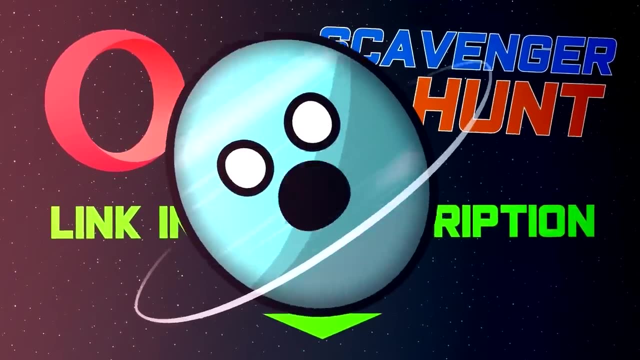 Okay, what are we waiting for? Let's do it. Also, if you want to join, use our link to download Opera and join the scavenger hunt while it's still going. We hope you can also be one of the winners. Now back to the video. 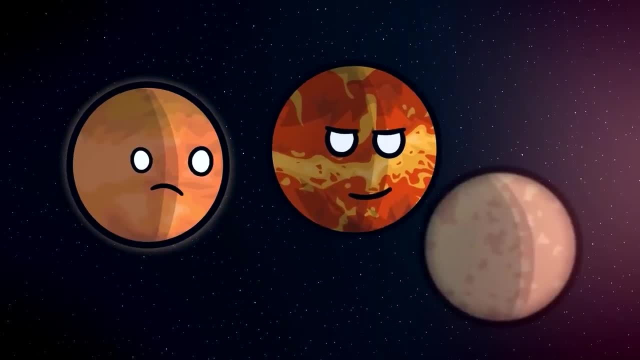 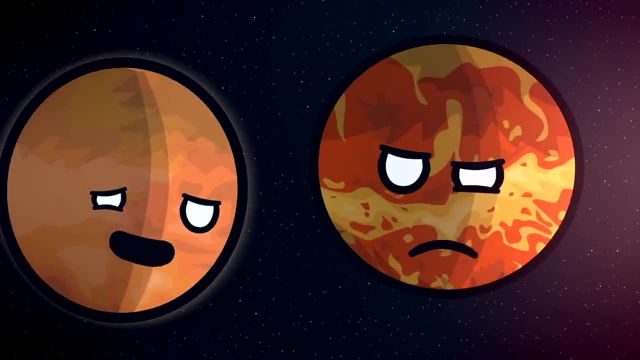 Hey Mercury, Hello Mars, Venus, What's up? Pipsqueak, Listen. We need to understand what happened to the Earth. Then ask him: Uh, we'd rather not Listen. the Earth went through a lot while you were gone and not all of it was nice. 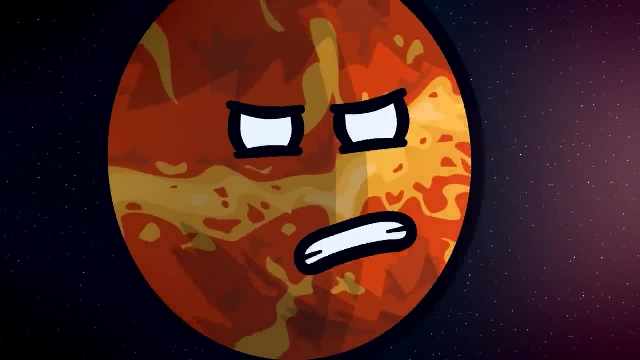 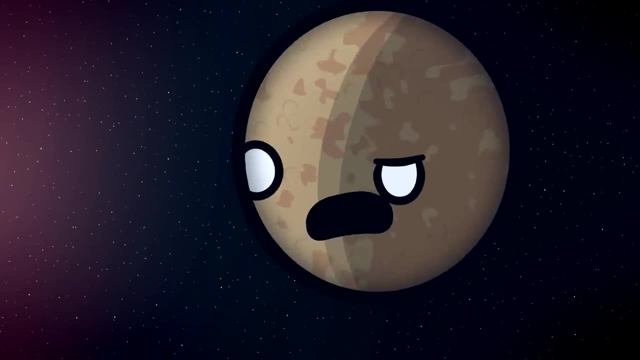 This is a conversation you need to have with him. Huh, Why are you being so annoying, Mercury? You're making this a lot harder than it needs to be. Hey, I wasn't part of whatever discussion you had with the Earth. 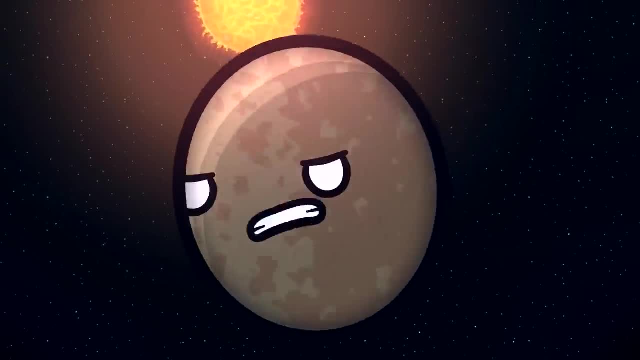 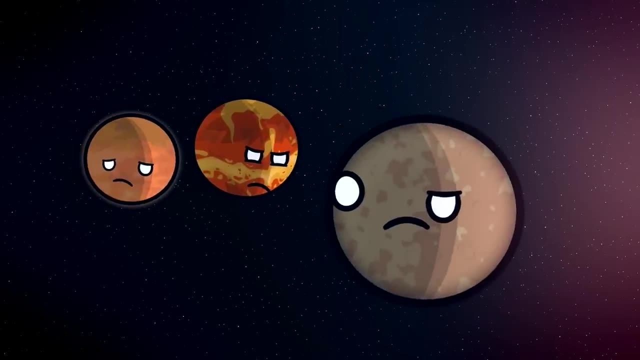 I've never been a part of anything you do, okay, So so don't come here demanding answers from me. He's right What You're right, Mercury, We haven't been fair with you. I mean, how did it come to this? 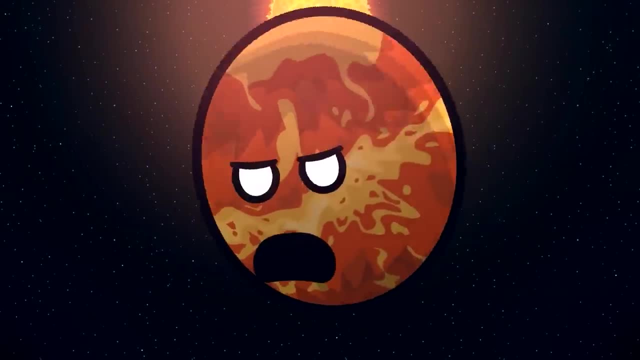 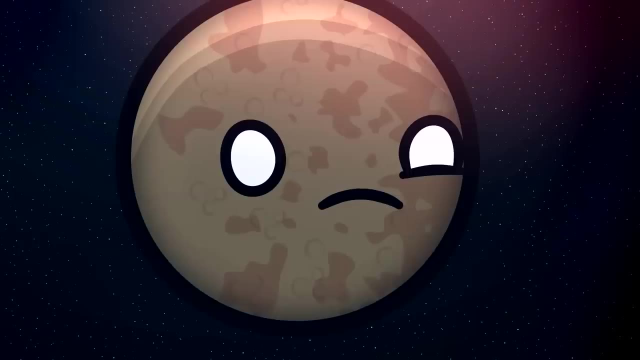 Come on, follow me. Do we follow him, or Ugh? Hello guys, What's going on? Everyone, we need to clear the air. okay, There's no air in Spar- Mercury. Sorry, Mars, everything is fine. 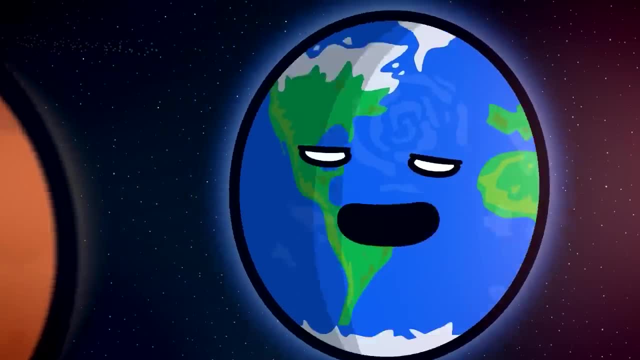 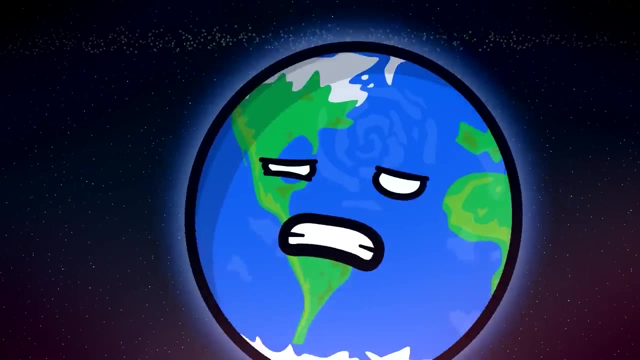 No Earth, none of this is fine, B-b-but I apologized, That's not it. It's just that Like, Are any of us really friends? Well, last time we talked No, before that, Me and you, you and Venus, Venus and Mercury. 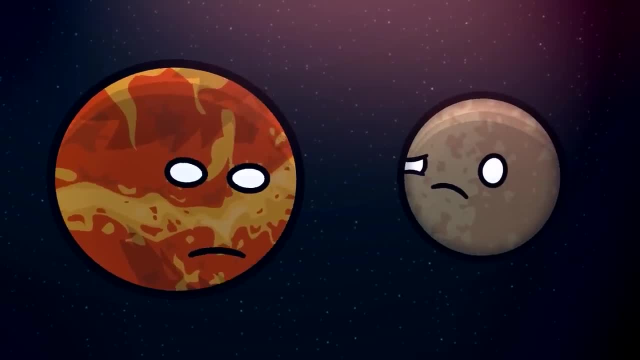 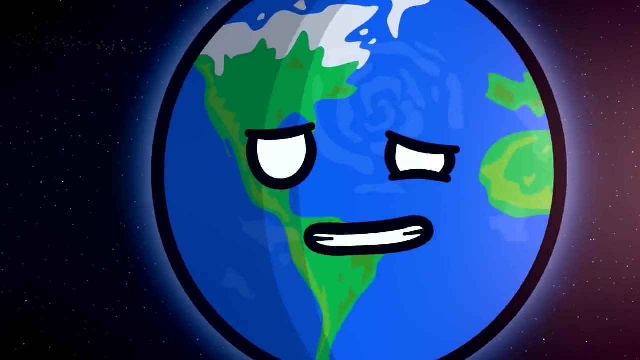 We are the rocky planets guys. That's pretty cool, right? So why are none of us like real friends? We Used to be friends, but then I screwed things up and Earth- it wasn't only you. 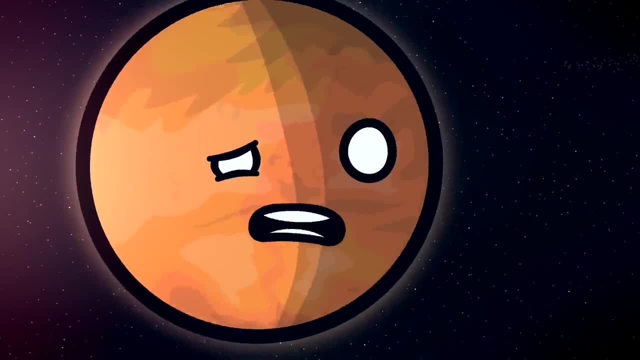 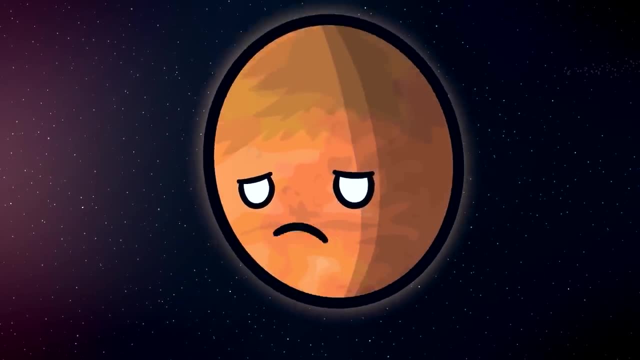 I also refused to pay attention to how you felt When you met Titan. I gave you a whole explanation of how Titan is so similar to you, And it never crossed my mind that you could feel insecure about it. It's not on you, Mars. 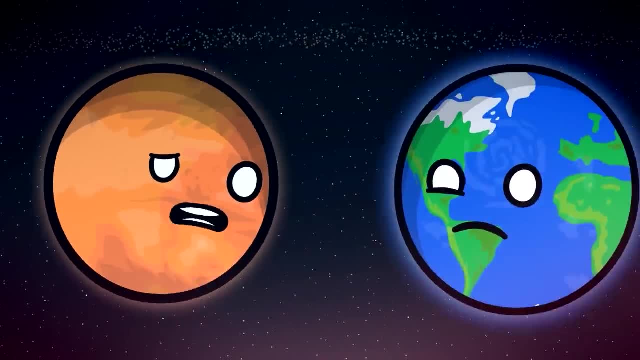 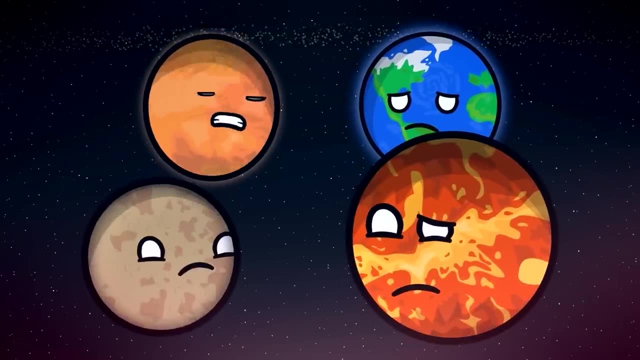 I can also be responsible for myself, Absolutely, But I was your friend. That's my point. We all have maintained such a Superficial relationship with each other, Even us Earth, Even us. I think you're exaggerating Mars. 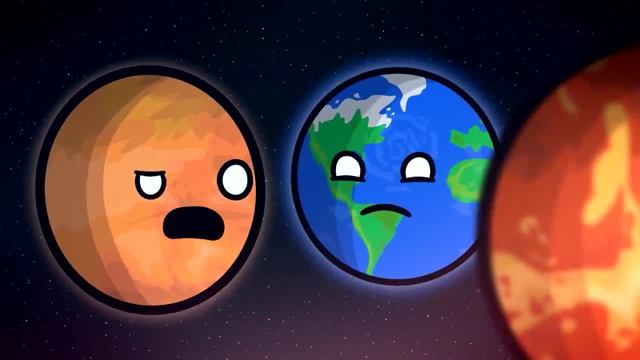 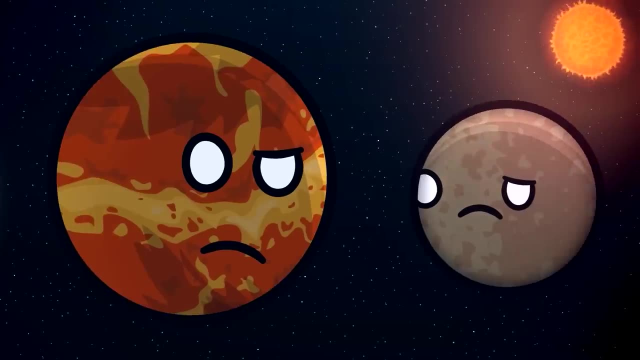 Am I? What about you? Venus, The Earth and you became friends just to spite me. You and I became friends And I became friends because we were fed up with the Earth And you and Mercury can barely stand each other. Okay, you do have a point. 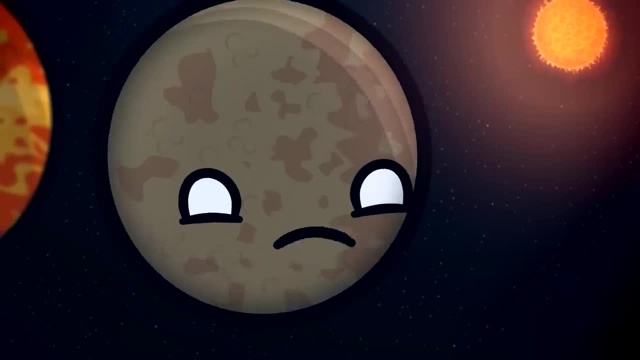 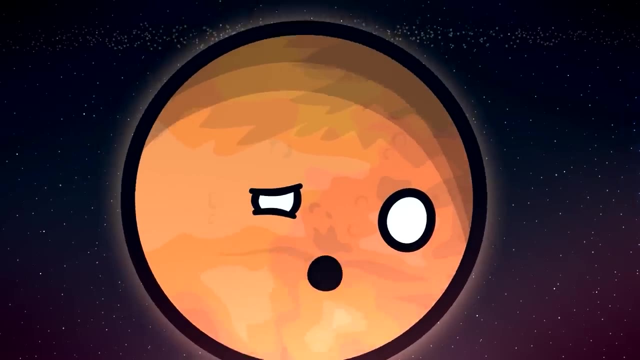 Mars. we've all known each other for billions of years. If we didn't manage to become real friends in that time, what can we do now? Maybe we've been too focused on the science of it all. The science of it all. 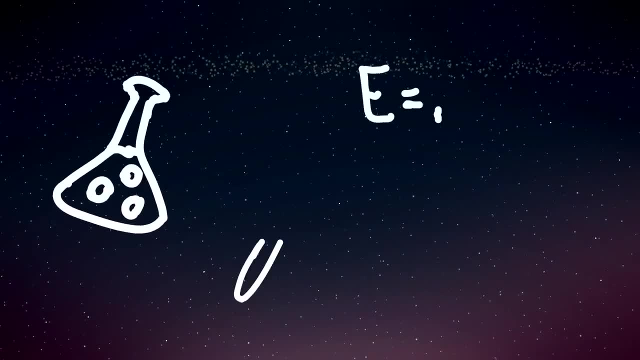 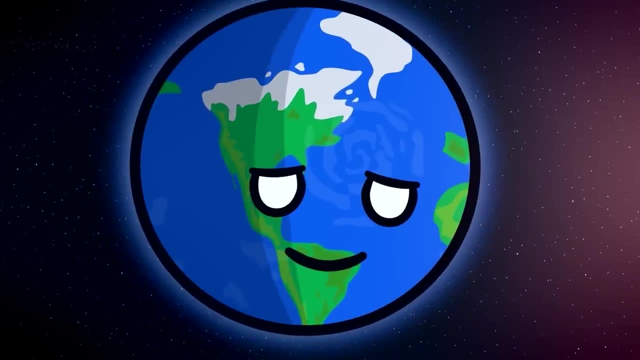 Yeah, We get so lost in discussing fun facts and science and how things are meant to work that we forget about what makes us Us. I think we should do both from now on. Ugh, this is a huge waste of time. I'm out of here. 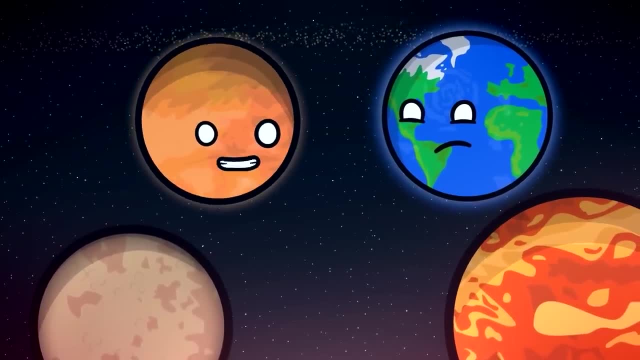 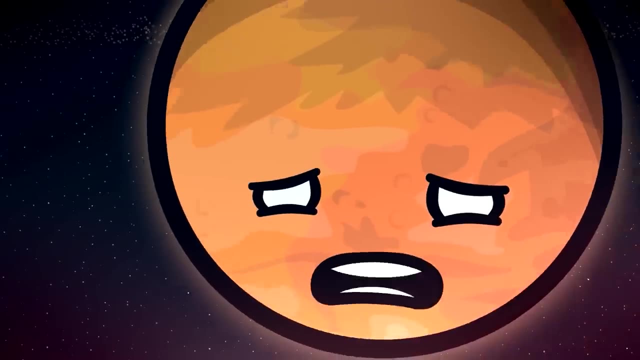 My name is Mars. I am the fourth planet from the Sun, orbiting between the Earth and Jupiter. My diameter is 4,217 miles, and I tend to think I know better than everyone else What You I Since. when do you? 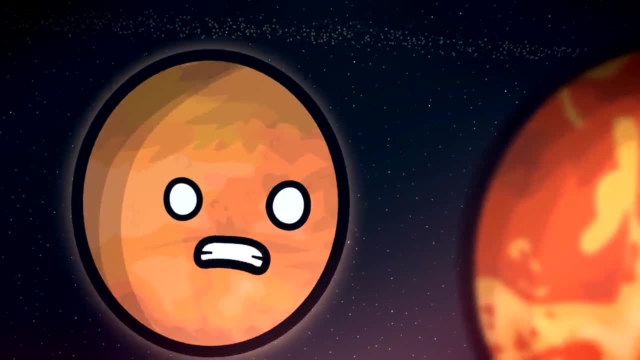 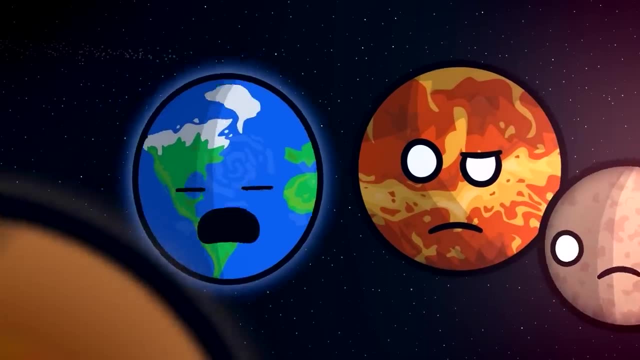 I don't know. I've always been next to Jupiter and he knows better than everyone. So, yeah, I tend to act as if I have the moral superiority, But I probably don't. Well, you do tend to be right most of the time. 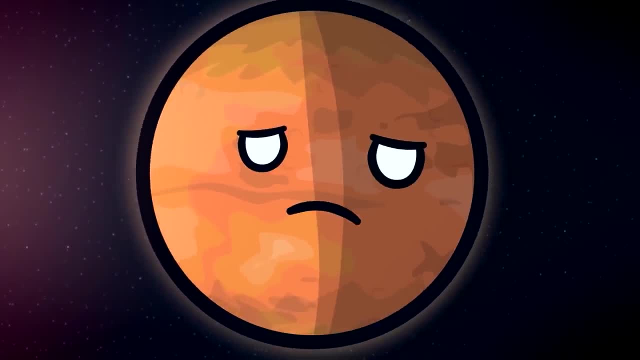 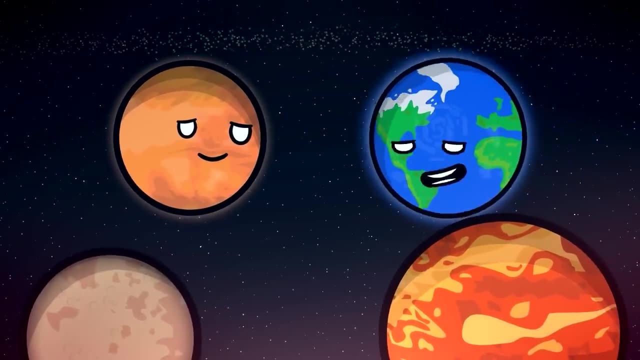 I know, I'm just saying that We got it. Mars, Thank you for sharing. I am the Earth. I am the third planet of the solar system, even if my Earthlings believed I was the center of the universe, or flat. 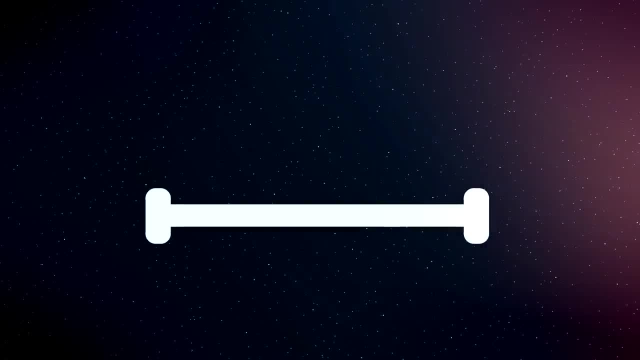 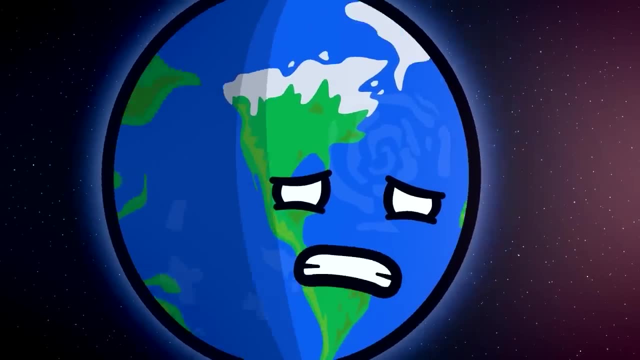 I orbit between Venus and Mars, My diameter is 7,907 miles And after everything that happened, I am afraid of the Earth. I'm afraid of being myself again. So that's what's troubling you. Yeah, I'm not sure which parts of who I am were the problem. 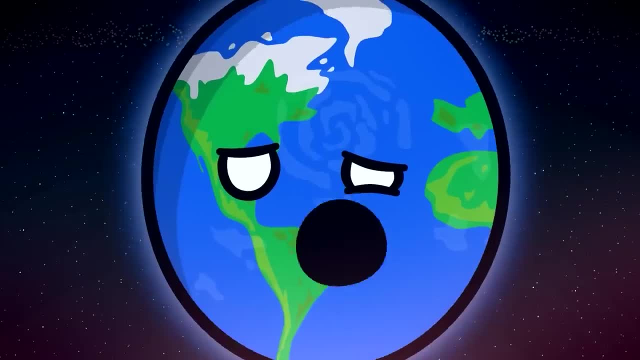 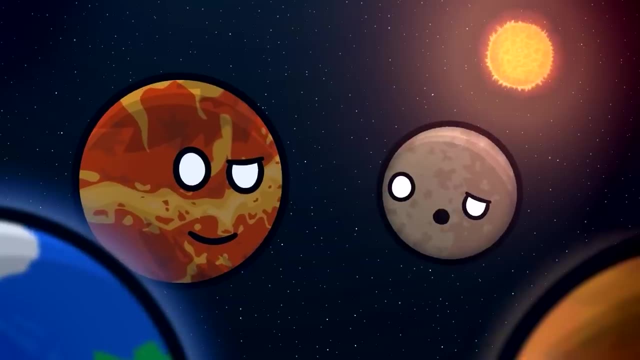 I don't want to say the wrong thing, or for you to leave me or to make anyone feel bad. What do you say? you try to be yourself, but with a bit more humility. That way, if you do something that is wrong, we can let you know. 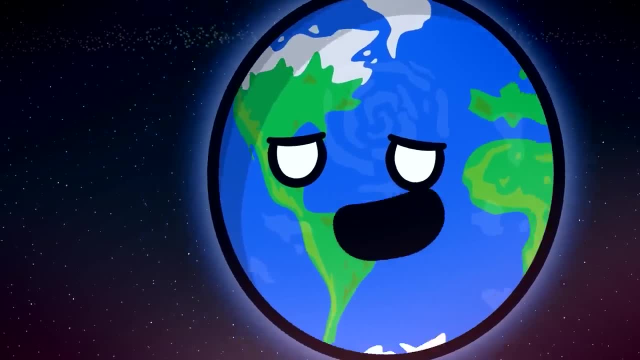 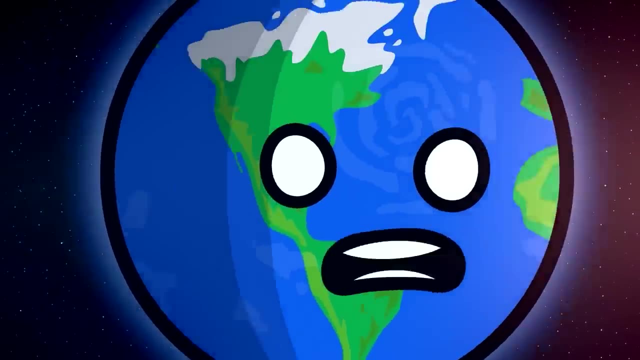 Yeah, Cheer up Earth. It's boring to see you all mopey and stuff. Thanks, guys. And does this mean I'm the best planet again? Earth, Nothing, Uh. OK, Venus, you're next. Do I really need to? 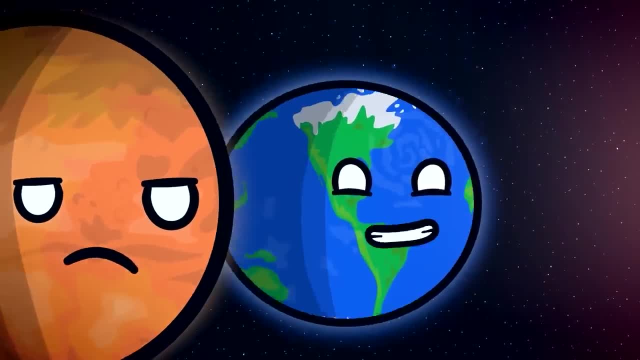 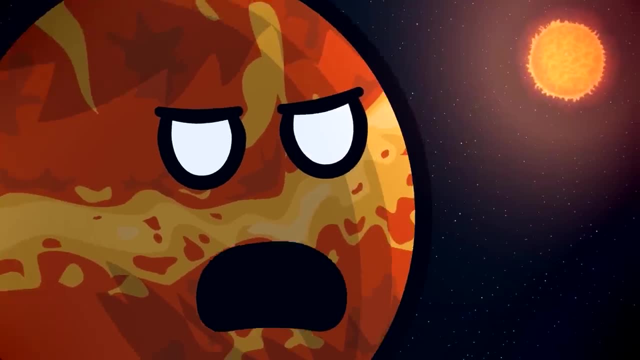 Come on, Venus, Everyone is doing it. Dude, you have to now, Don't leave us hanging Fine. Hello, I'm Venus, second planet from the sun, between little pipsqueak over here and the Earth, 7,500 and something miles of diameter. 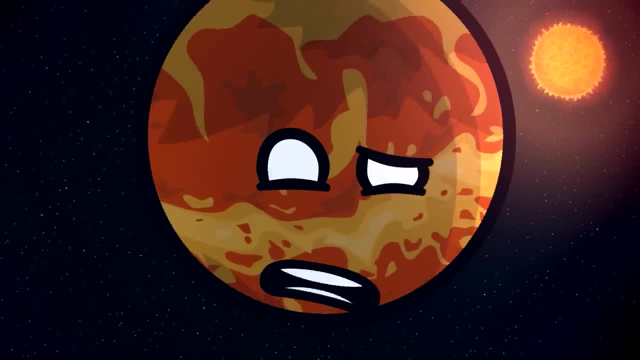 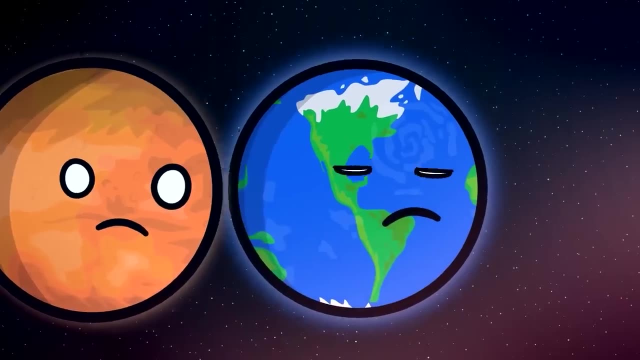 And I, well, I don't know, I don't like my orbit at all, or my atmosphere, or myself. all that much Venus. OK enough, Your turn, Mercury. Uh, hello, I'm Mercury. I'm the first planet from the sun, which means my neighbors are the sun and Venus. 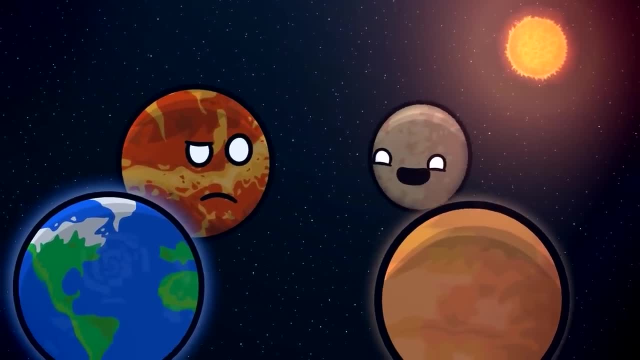 My diameter is 3,032 miles And I I don't like being the smallest planet. I'm afraid of becoming like Pluto and getting kicked out of the planet club. Oh, come on, dude, That is not going to happen.